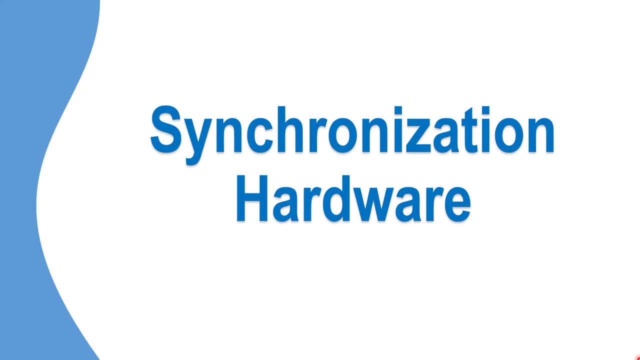 In the last video lecture we have seen the software-based solution to the critical section problem that was using Peterson's solution. In this video lecture we will see the hardware-based solution to the critical section problem. with the help of locks, Race conditions are prevented. 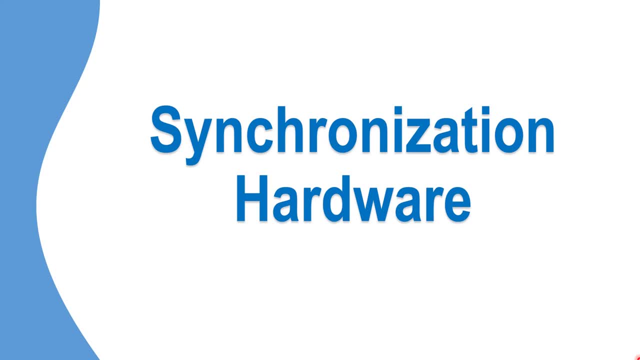 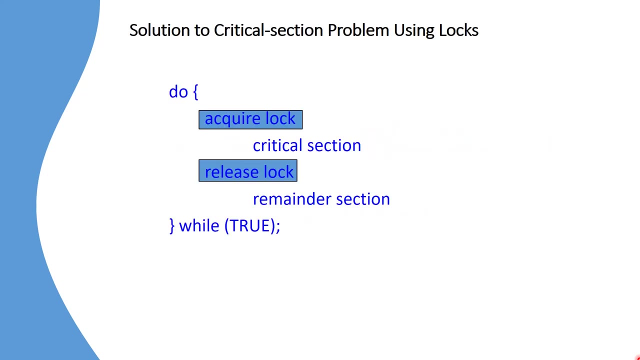 by requiring the critical regions to be protected by locks. That is a process must acquire a lock before entering a critical section. It releases the lock when it exits from the critical section. So let us look at one example. So in this example there will be multiple processes. 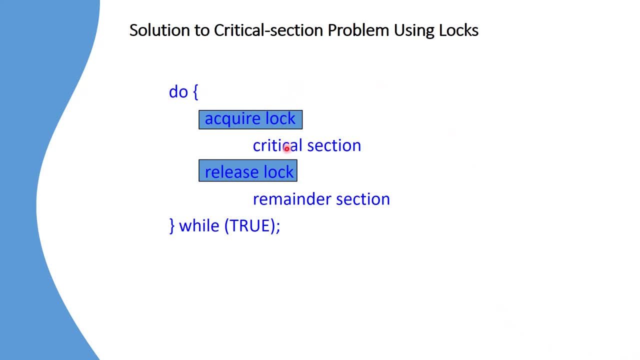 that will be willing to enter the critical section, But a process will be allowed to enter only after acquiring the lock. So even though there are multiple processes- P1, P2,, P3, P4,- there are multiple processes that will be willing to enter the critical section. So 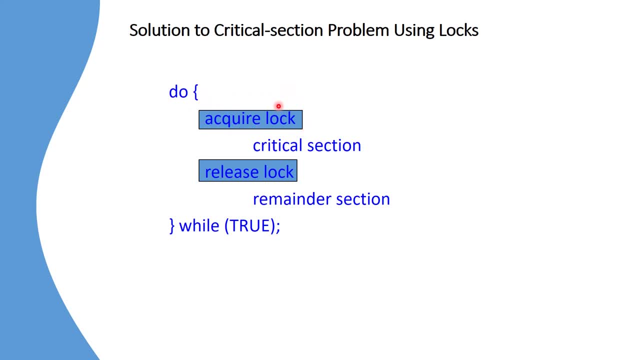 there will be only one process that will be allowed at a time to acquire the lock. So once the lock is acquired by the process- for example, if we consider the process P1 acquires the lock, it will enter the critical section, While other process will wait for the lock to. 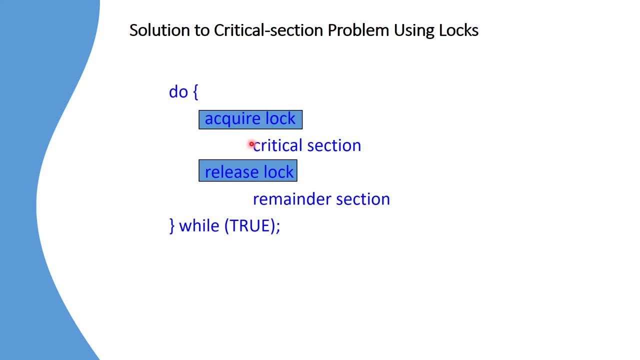 be released by P1. So once the process P1 has executed in the critical section and when it comes out of the critical section, it releases the lock. Once the lock is released, the other processes which were waiting can now compete among themselves. 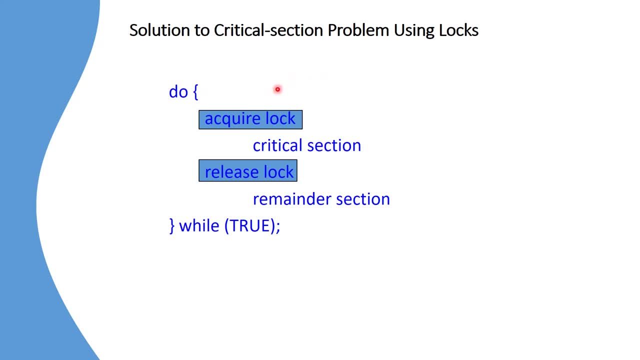 to acquire the lock. So a new process will be given the chance to acquire the lock. So that is how the locks are used in the solution to the critical section problem. We can understand this using one more example, real life example. 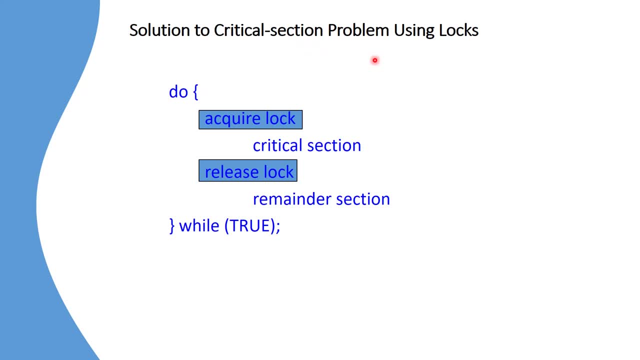 We can consider there are multiple faculty or multiple teachers competing for a class. Now one of the faculty is able to enter the class, So once he enters the class he locks the door. So once the door is locked, other faculty members cannot enter the classroom. So that is how. 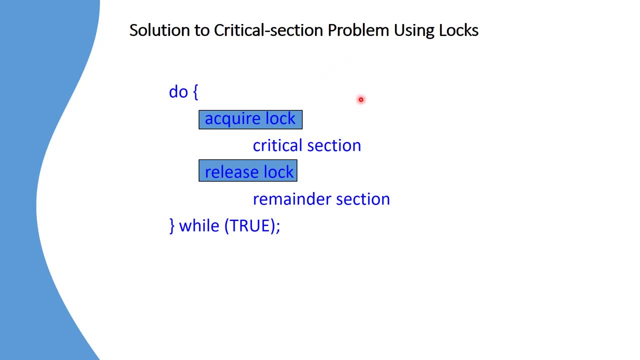 acquiring the lock by a process is similar to locking the door of the classroom by the faculty who managed to enter the classroom. So once the class has been taken for the duration of the time, then the faculty will unlock the door or the faculty will release the door. This is similar to the 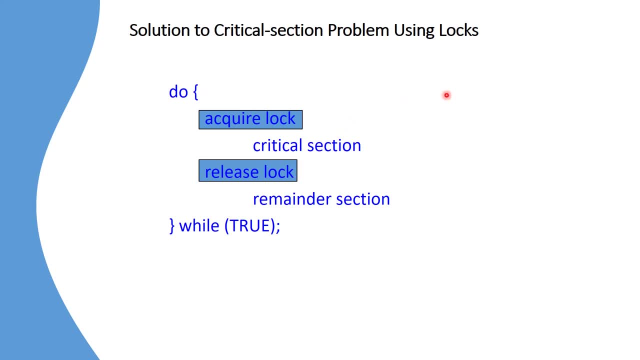 process releasing the lock. So now the faculty members who were waiting outside the class can now compete among themselves to acquire the lock That is among them. one of them will go inside the class and again follow the same process by locking the door. So 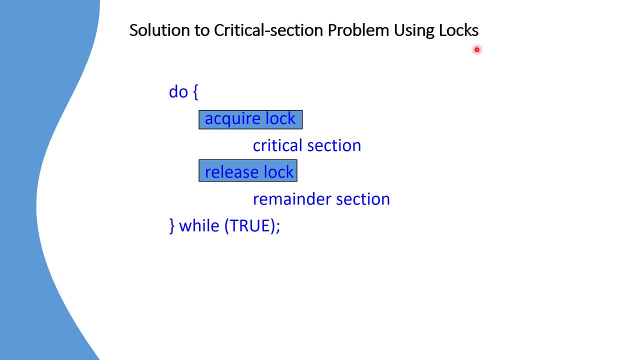 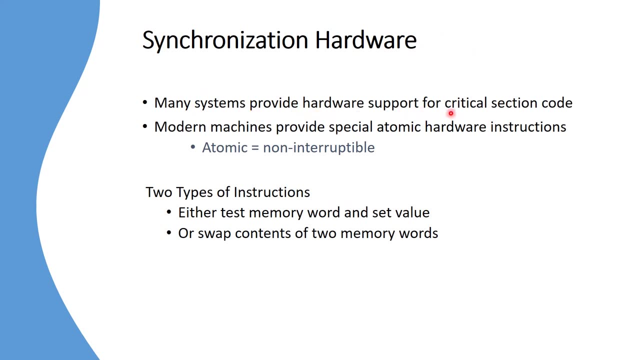 other process won't be able to enter. So this is similar to the solution to critical section problem using locks. So many systems provide hardware support for critical section code. Modern machines provide special atomic hardware instruction. So we'll see today two hardware. 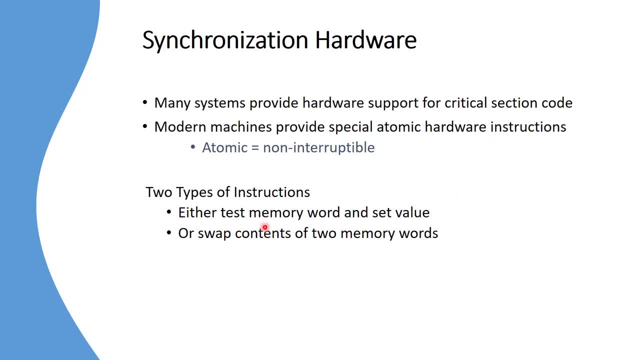 instruction One is test and set, that is, test memory and set the value. So here we will test the value of the lock variable and set the value. that is one atomic instruction. and the second atomic instruction is swap, the contents of two memory words. now the two instructions are atomic means. when they are executing or a process is. 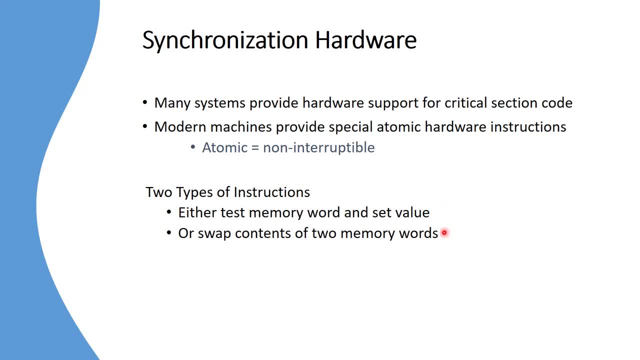 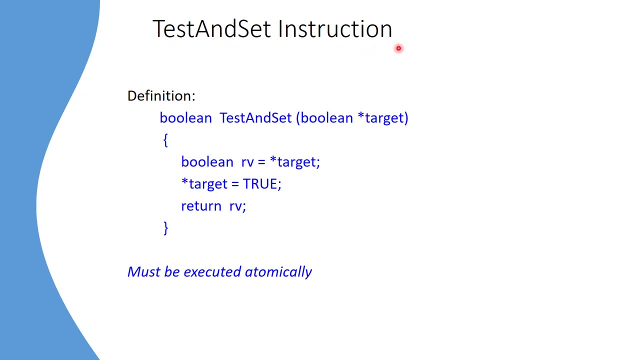 executing any one of these instruction. other instruction cannot interrupt in between, that is, it is non interrupt table. so to understand more about this, let us look at one example. so we are looking at the test and set instruction. so this is the hardware based solution to the critical section problem. now, if you see, the test and set function has a Boolean variable target. so 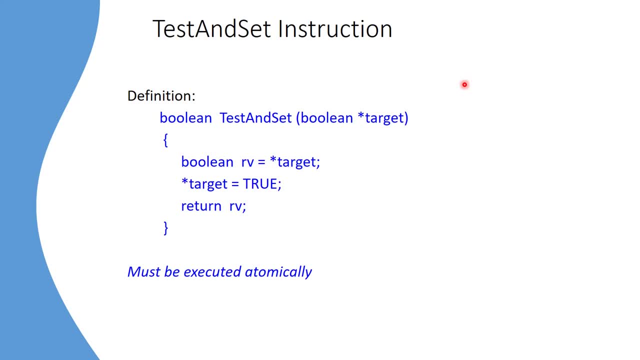 it will read an address, take the value from the address, the Boolean value, and stored in target that value. value is the value of the case value and this is the value of the test and set function. value is passed to the variable RV, the target value. it will be changed to true, true value. 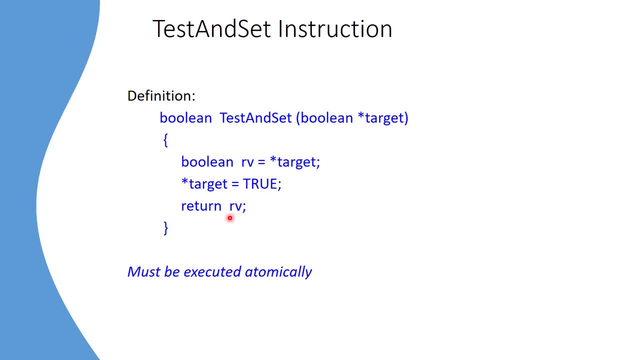 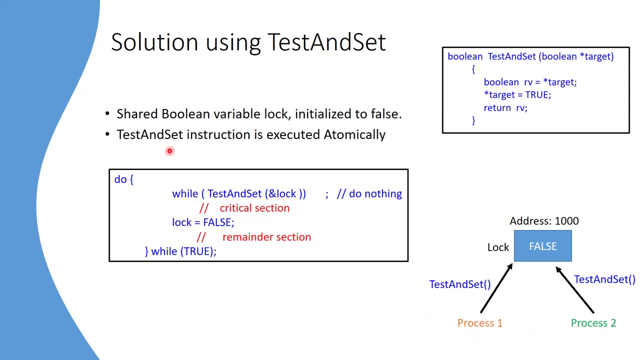 And whatever it has been saved in the previous line will be returned. Now, if we look at this particular example, we see that there are two process, process one and process two. both of them are executing this particular code Initially the log. the log variable is set to false. 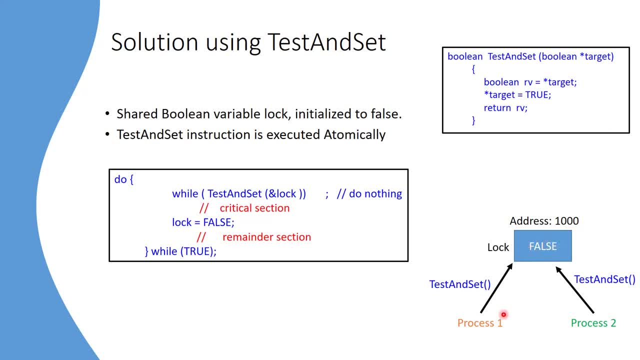 The log variable is stored in address 1000 and is set to false, and both process one and process two is executing test and set operation, And this is atomic. As the operation is atomic, only one of them will be allowed to execute the instruction. 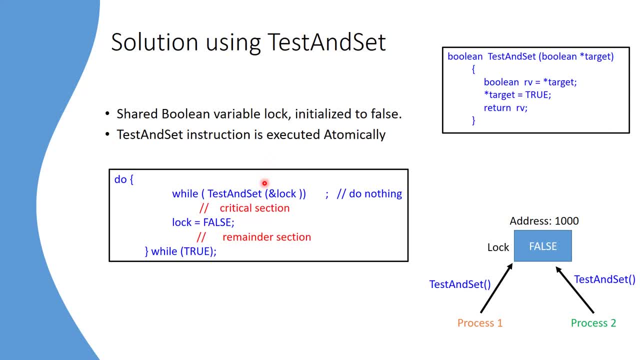 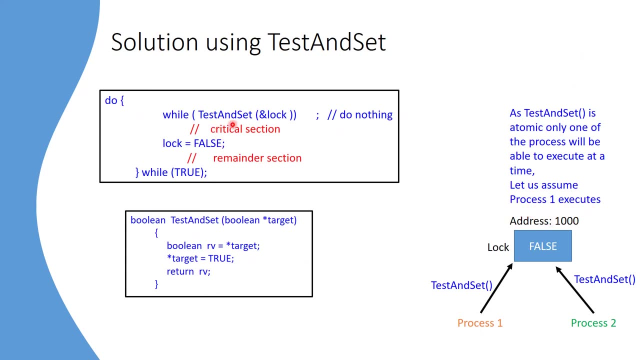 not both. So both the process wants to execute this instruction, but there will be only one process that will be allowed to enter. So, as for an example, let us assume that process, one process, one executes the test and lock instruction as the value or the initial value of the log variable is false. 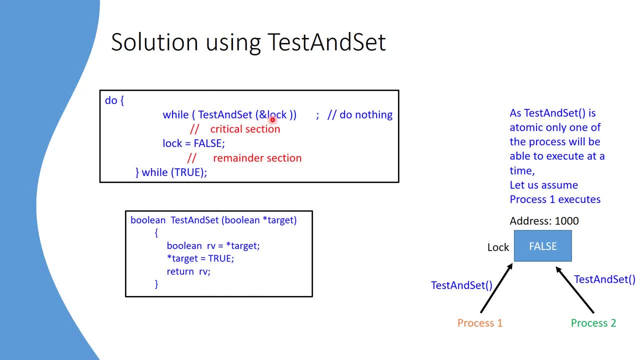 So it will test while test and lock ampersand lock. So address of lock. so address of lock is 1000, it will pass the address of lock to this variable target, So target will read whatever is at this location: 1000.. 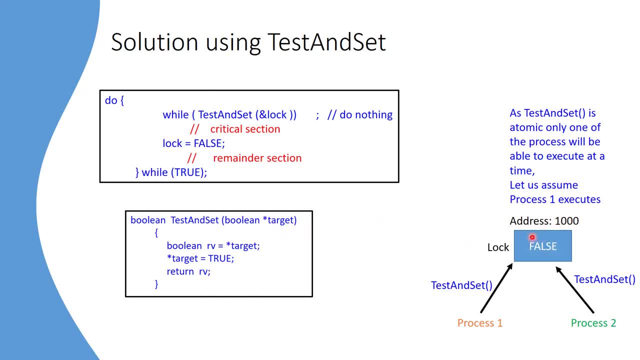 So we see that the value of target is false, which is the initial value. So process one. checks that the value is false, So process one will enter the critical section. Now process one what it does: it change the value of target to true. 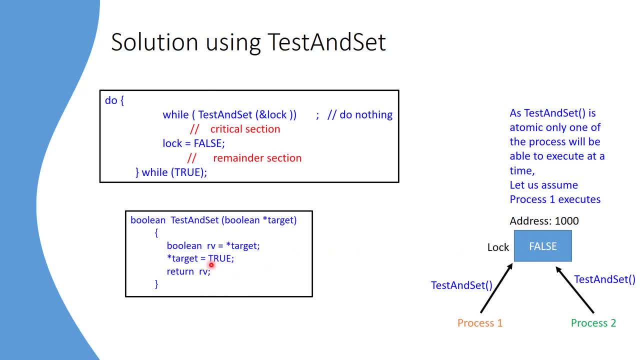 Initially the value was false. it's changed the value of target to true. Now the log variable contains the value true. Initially it was false. Now it contains, or it is changed to true Now, once it has been changed to true. process two checks the value of the log variable using: 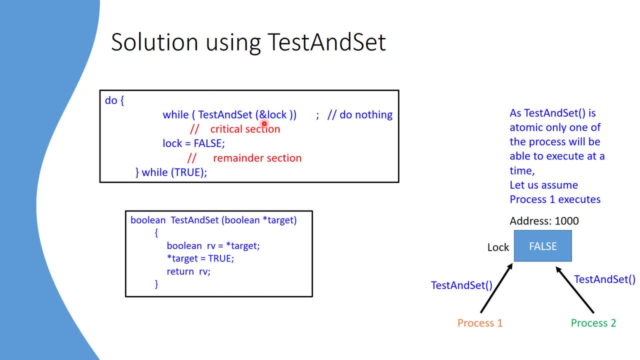 test and set instruction and it sees the value is true. So process two will go in an infinite loop or it will do nothing. So process two checks the value of the log variable using test and set instruction, and it sees the value is true. Now process one checks the value true and it is weighting to true. 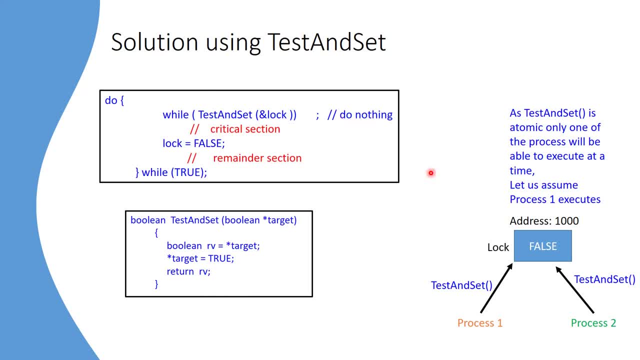 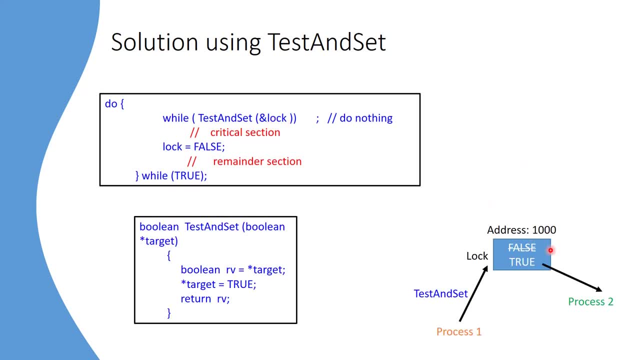 Now it is weighting to true. Now we can also check If the log variable is true or not. So process two checks the value is true, It is weighting. or we can also say it will be busy waiting. So process two cannot enter that critical section because the log value is set to true. 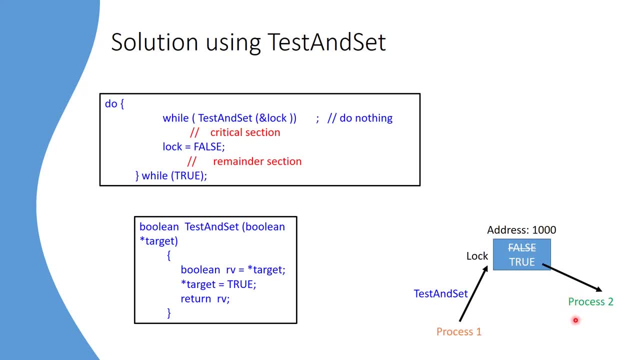 So log value is changed from false to true. So process two is waiting, busy waiting, while process one is inside the critical section. So this also satisfy the condition of mutual exclusion, where we understand that only one process will be allowed to enter. So for the first column of the problem we can also check. 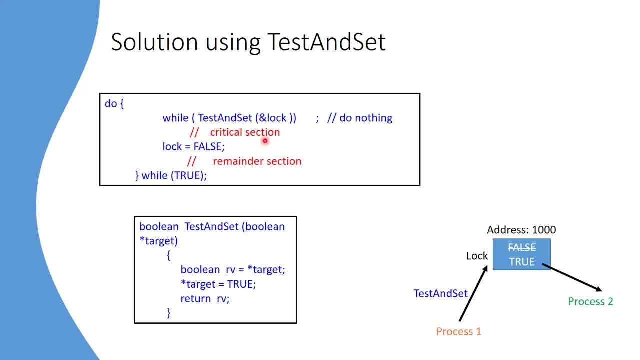 And let's check the critical section. So here, process one reads the value which was initially false, change it to true and enters the critical section. In the critical section it executes the code. and when process one comes out of the critical section, it changes the log variable to false. 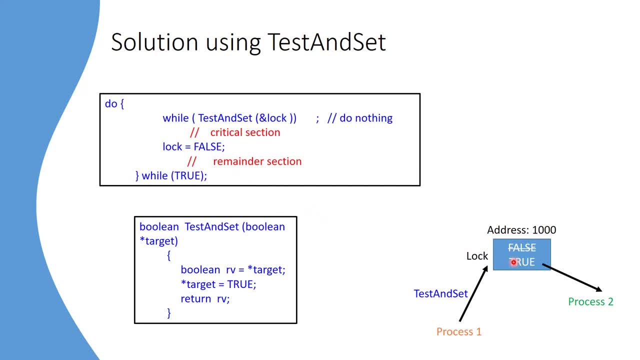 So from true. then it is again changed to false. So once it has been changed to false, now process two, which was initially not able to enter or that was busy waiting, now sees that the log value is false. Now process two can enter the critical section. So that is how two processes both. 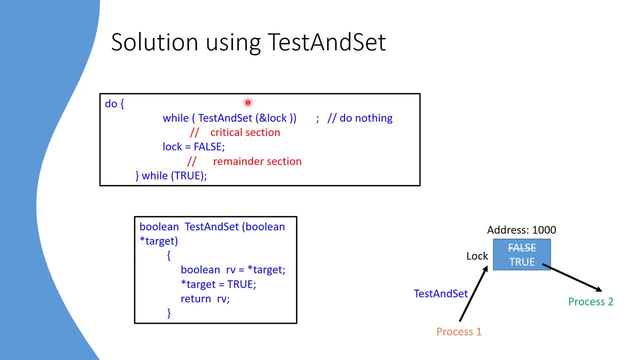 compete But being the operation atomic, only one of them will be executing this one. So when the process is executing this one is changes the log value from false to true, so other processes are not able to enter the satisfying the mutual exclusion. Let us look at the second. 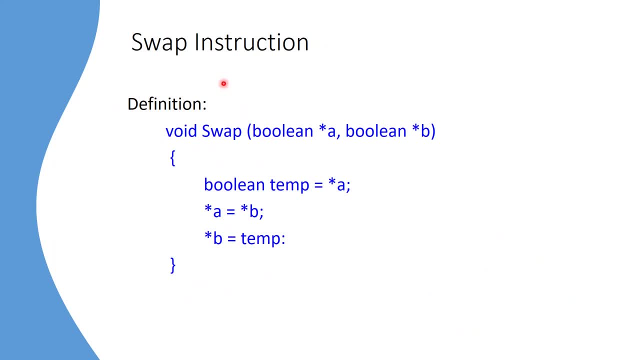 operation which is swept. so there are two boolean variables, A and B, And if you see the values are being swept: E value is given to B and B value is given to A. So that is when the process of executing it changes the log value from a to Z. There is a. big decentralization happening here. So to make sure that this comes true, any time the process is not supplied And when the process is executed, this one is changed from false to true, So other processes are not able to enter, thus satisfying the mutual exclusion. Let us look at the second operation. 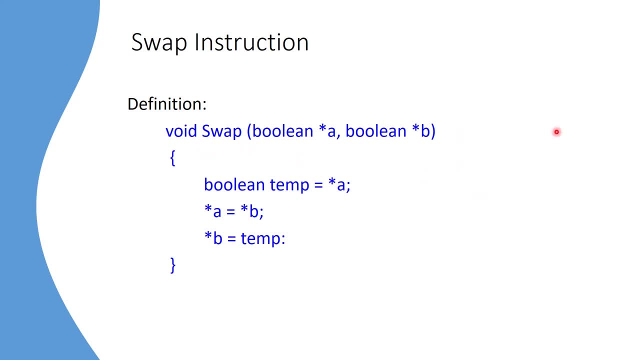 the swap operation and again, this operation is atomic. that is, if two processes or multiple processes are trying to execute this, all of them will not be able to execute it simultaneously. only one process at a time will be able to execute, and while the process is executing this set of instruction, other process has to wait. they cannot interrupt. so if we look at this, 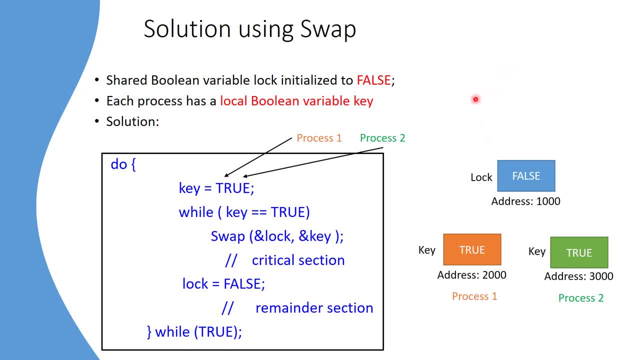 particular example, we see that there is a log variable which is initialized to false. so we see that in the address 1000, the log variable which is initialized to false. so this is the global variable. each of the process, in this example process 1 and process 2, have their own key, which is a. 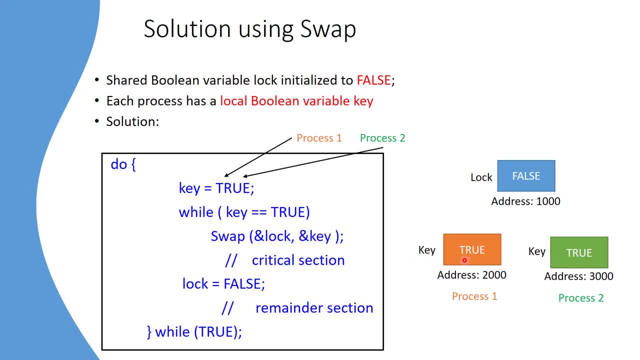 local variable. so process 1, the local variable key, is set to true, and process 2, the local variable key, is also set to true, and they are stored in address 2000 and 3000 respectively. now this particular code is executed by both the processes, so initially the key is true. 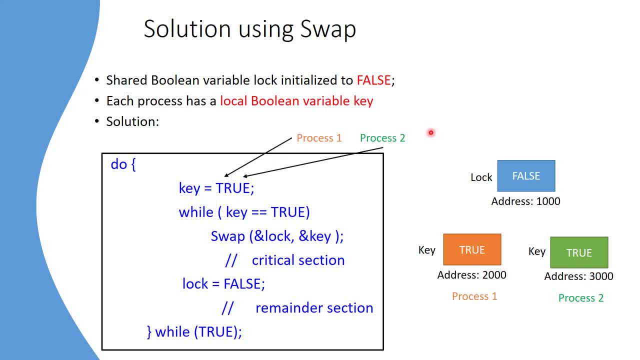 for process 1 and process 2. both of them, both the process process 1 and process 2- the key value is true. now, if the key value is true for both of them, this particular statement will be executed. now again, we have seen that this particular operation is atomic. that means only one of them. 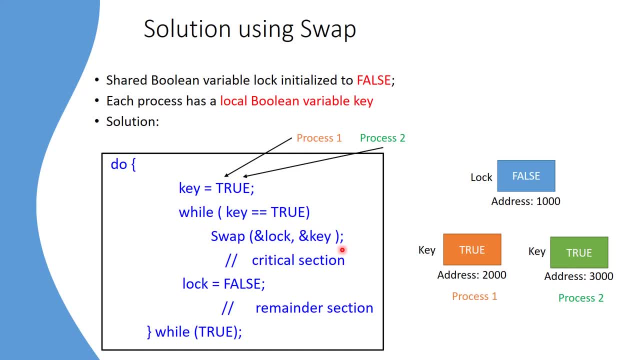 will be able to execute the operation, so we assume that process 1 is able to execute. so when process 1 is executing this, it is passing the address of lock and address of key, so process one, the address of lock is one thousand and address of key is two thousand, so one. 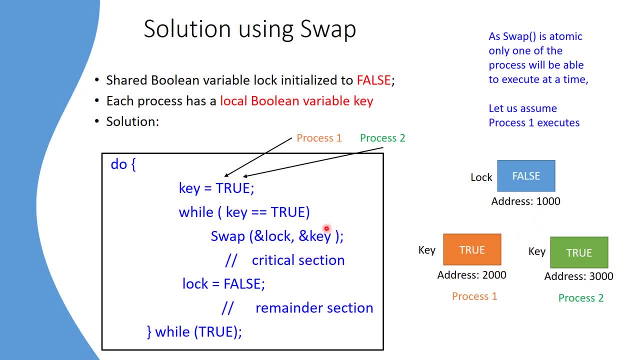 thousand and two thousand is passed to this particular instruction now, because the key value is true. it is repeated in this particular line. only now, the swap variable: what it will do? it will swap the value of lock and key, so log value is false and key value is true for process one, so it will interchange the values. 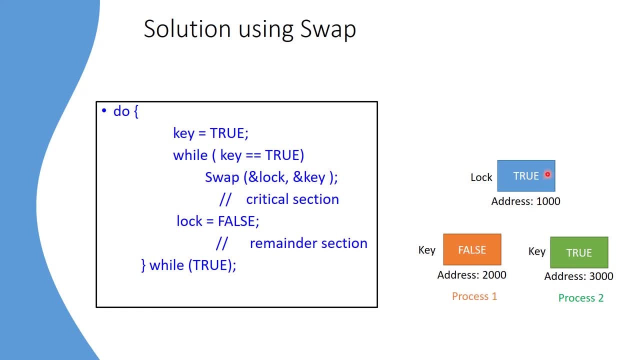 so we see that it is changed from false to true and it is changed from true to false. so once the values are changed, key value becomes false. so as false is not equal to true, process, one is able to enter the critical section. i will repeat: once the swapping is complete process, one is able to enter the critical section. 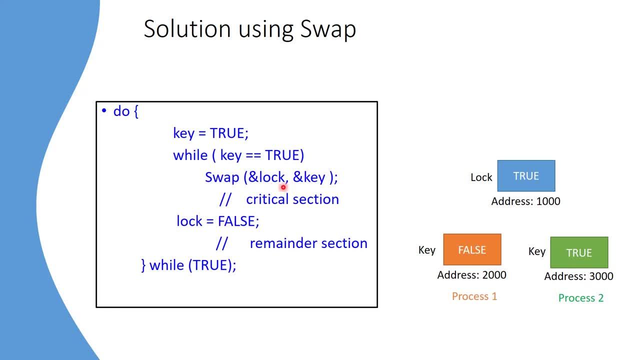 i will repeat: once the swapping is done, the key value is false. if you see here, the key value is false. so once the key value is false, process one able to enter the critical section because this condition is false. so it enters the critical section. now process one: is not executing the swap. 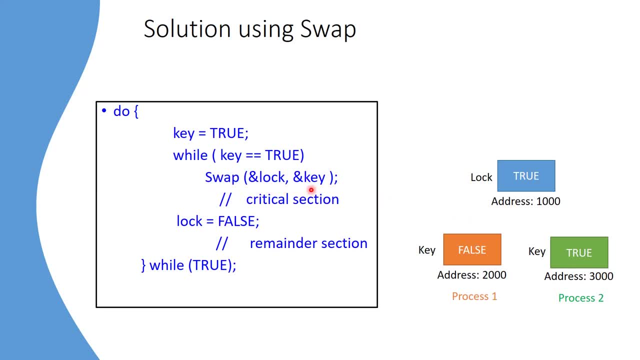 instruction. so process two can execute the swap instruction now. process two passes the address of the lock, which is 1000, and the address of the key, which is 3000. so 1000 and 3000 is passed. accordingly, the value is true and true, as the value is true for both the cases. 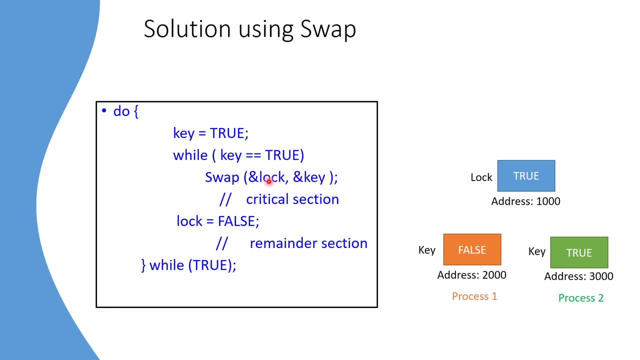 even after interchanging, swapping, the value remains true, only so true. so the condition for process 2 is true, is equal to true. so the condition is true. so process 2 waits in this particular section of the key. so all goes in an infinite loop, Whereas process one, which entered the critical section, 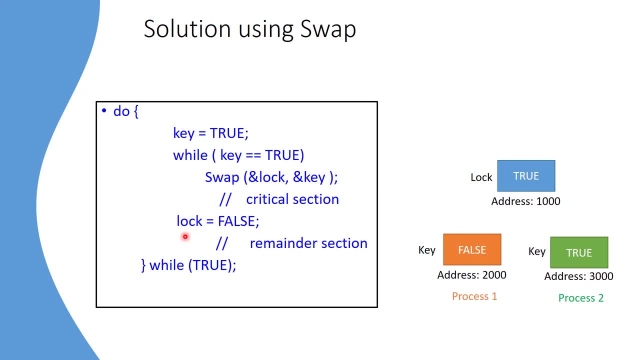 executes the code and when it comes out it changed the log variable to false. So process one. when it comes out, is changed the log variable from true to false. Now process two, which was in this particular section, busy waiting, So process to sees the value of lock variable. 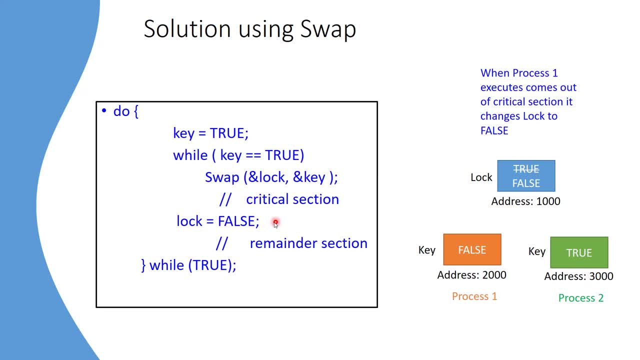 change to false at this particular line by the process one. So process to see that false is not equal to true. So it goes to the critical section and executes the code in the critical section. So we see that this particular swap operation also satisfy mutual exclusion when, when one. 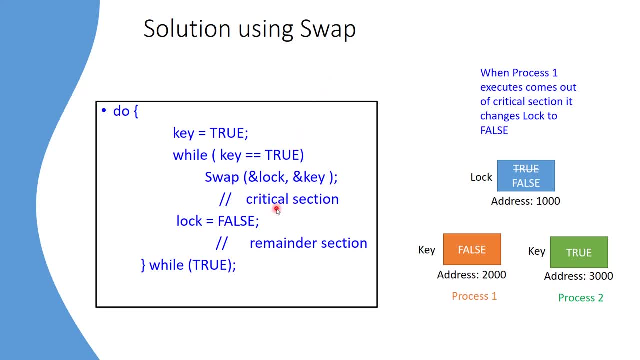 process is inside the critical section, it changes the log value from false to true so the other process cannot enter. similarly, when the process comes out of the critical section it again changes back it to false, so a new process which wish to enter now can enter. so only one process at a time is allowed to enter in the critical section. so we have seen. 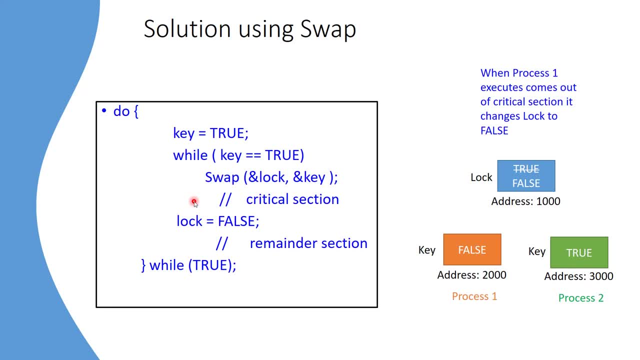 the two solution, one using test and set and another one using swap. so both the operations are atomic and they satisfy mutual excretion. however, they do not satisfy satisfy bounded waiting. that's all for now.